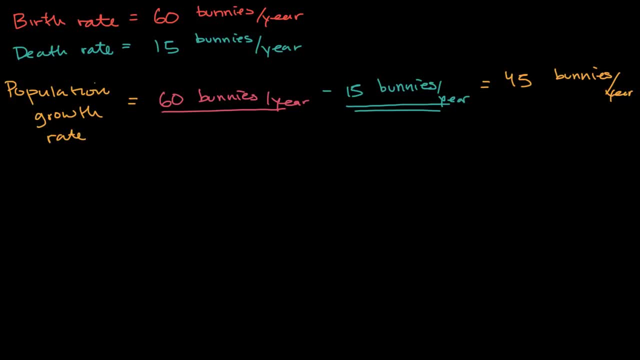 And to put that in the language of your AP Biology formula sheet, the notation they use for population growth rate they use a fancy notation. So actually let me just write it over here. They say n is equal to your population, n is equal to population. 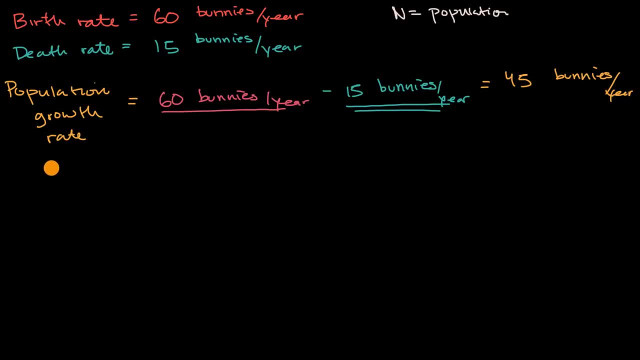 and then your population growth rate. they use calculus notation, so our change in population per change in time. This is really talking about something in calculus known as instantaneous change, but we don't have to get too bogged down with that just yet. 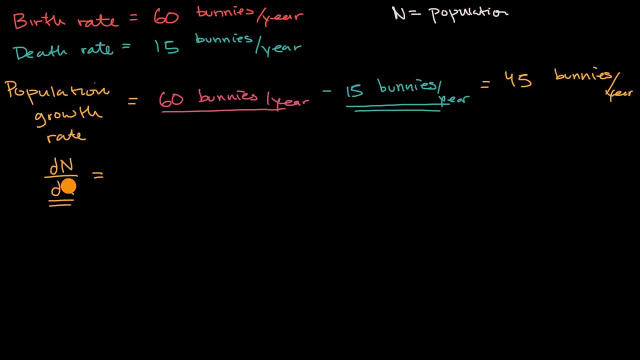 But your population growth rate, which you could use this notation for, is equal to your birth rate, 60 bunnies per year, and the notation they use for birth rate is just b. They don't use the same rate notation for that. 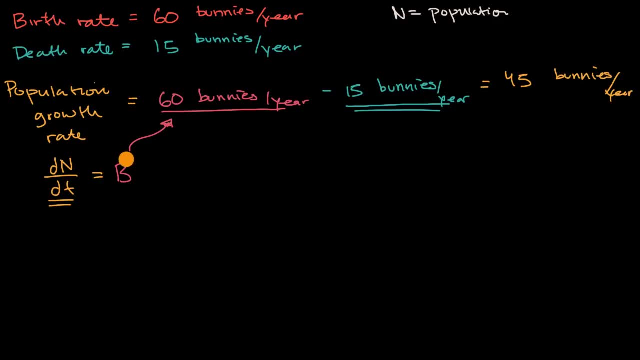 I probably would have. but that's fine, I'm just trying to make you familiar with what you might see. And then minus the death rate, minus d. So this right over here is something that you would see on that formula sheet, but it makes fairly intuitive sense. 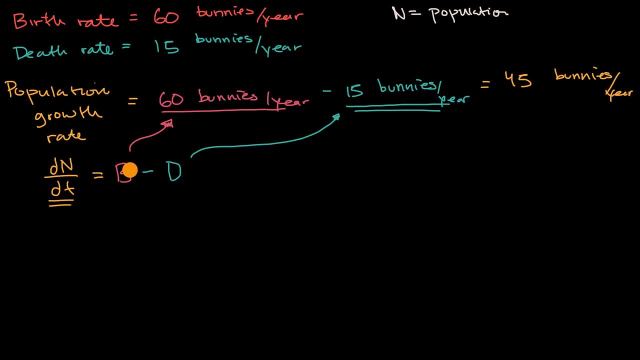 Now the next idea we're going to talk about is, or we're going to think about is something known as a per capita growth rate of population. Let me write it out in words first. So here we're going to think about a per capita growth rate, or population growth rate. 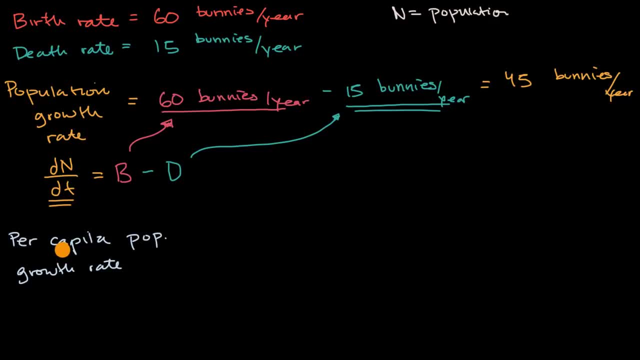 per capita population growth rate. Now, per capita means you could view it as an on average per individual. What is the average growth rate per individual? What is that going to be? Pause this video and try to think about it. Well, one way you could think about it. 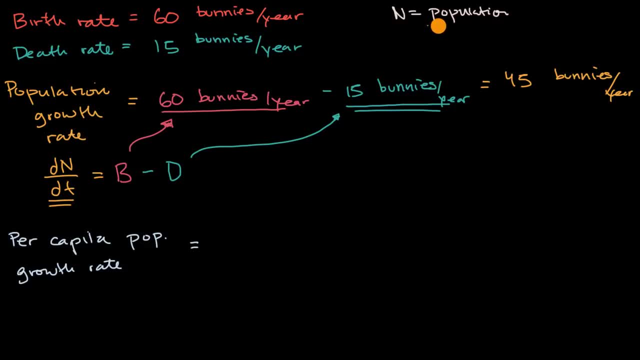 it's the total population growth rate divided by the population, divided by the number of people there are. So it's going to be our population growth rate, growth rate divided by, divided by our population population. Now let's say that we have a population of 300,000.. 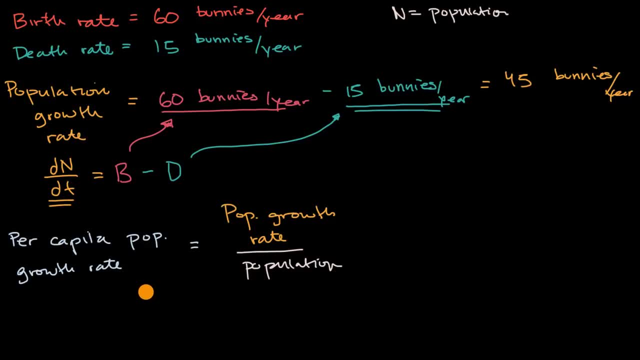 Let's say we have a population of 400,000 bunnies. Actually, let's make the math a little bit simpler. Let's say we have a population of 450 bunnies. So what is going to be our per capita population growth rate? 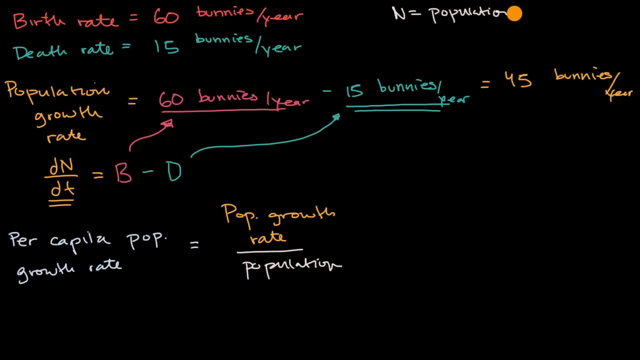 Pause this video and try to figure that out. Well, if we have a population of 450 bunnies, 450 bunnies, our population growth rate per the number of people we, or number of bunnies, I should say. 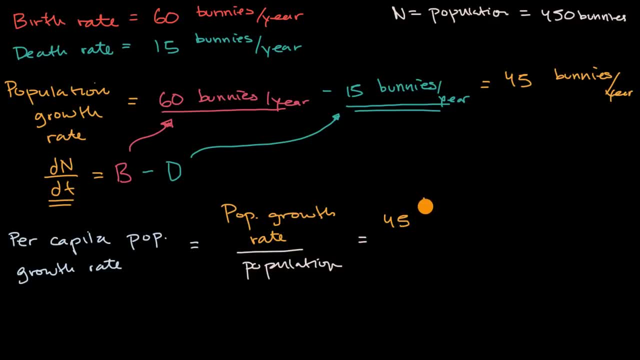 is going to be equal to our per capita population growth rate is 45 bunnies bunnies per year, and that's going to be for every 450 bunnies. 450 bunnies, which will get us to 45, divided by 450, is 0.1,. 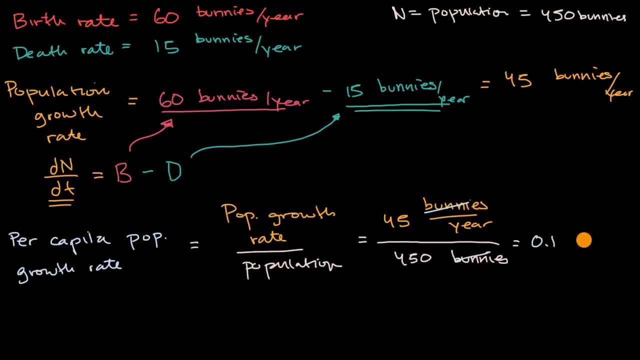 and then the units bunnies cancel with bunnies, so it's 0.1 per year. Now why is per capita population growth rate interesting? Well, it tells us just how likely, and in most populations you need at least a male. 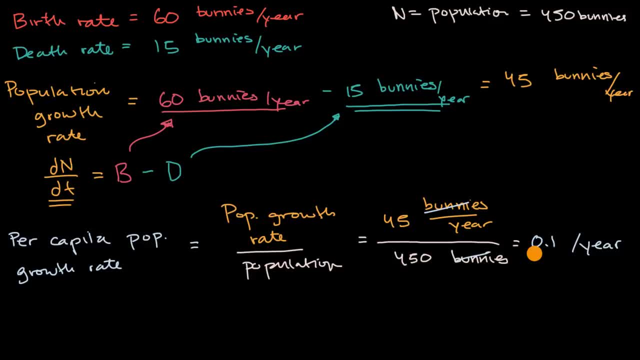 and a female in order to reproduce, but there are some organisms that can just split and reproduce asexually. but it tells us on average per individual organism how much are they going to grow per year. So it gives you a sense of that. 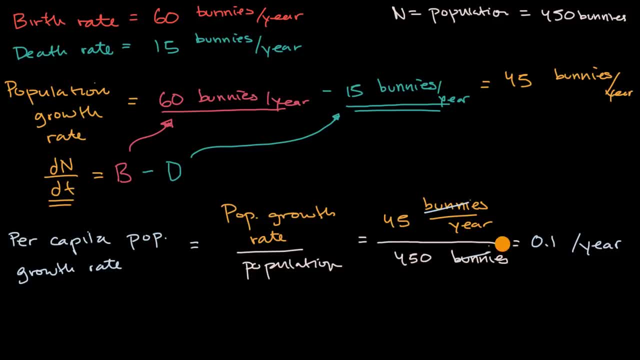 Now connecting it to the notation that you might see on an AP Biology formula sheet. it would look like this: The per capita population growth rate is usually denoted by the lowercase letter R, And then they would say that that is going to be equal. 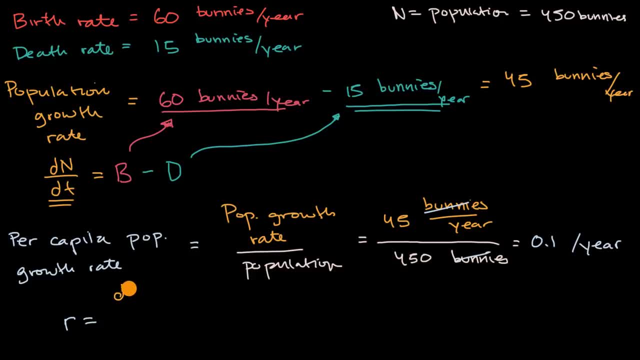 to our population growth rate, which we've already seen. that notation, the rate of change of our population with respect to time, Dn Dt divided by our population, divided by our population. Now we can algebraically manipulate this a little bit. 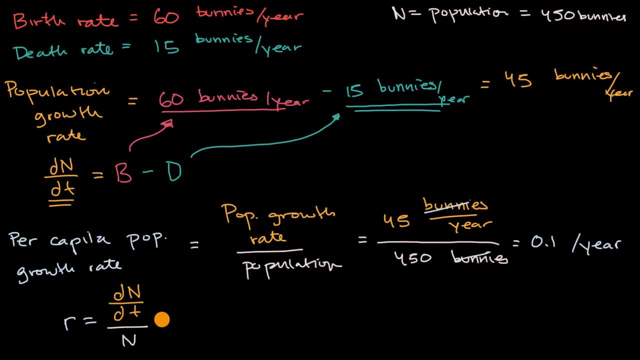 to get another expression, we could multiply both sides times our uppercase N times our population, And we're going to get dN dt is equal to N times R or R times N. Let me rewrite it. We could rewrite this as dN dt. 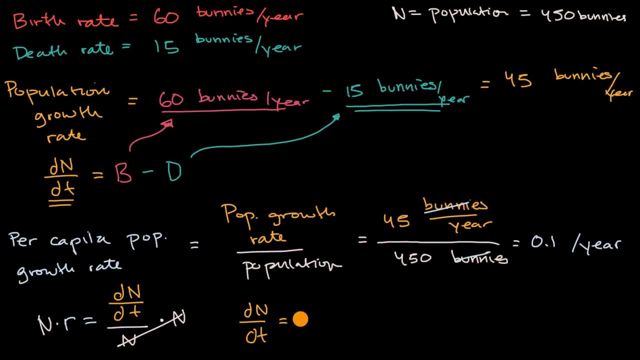 is equal to our per capita population growth rate times our population. Now this once again makes sense If you say: okay, this is how many people, how many individuals I have, and if in a given year they grow by this much on average. 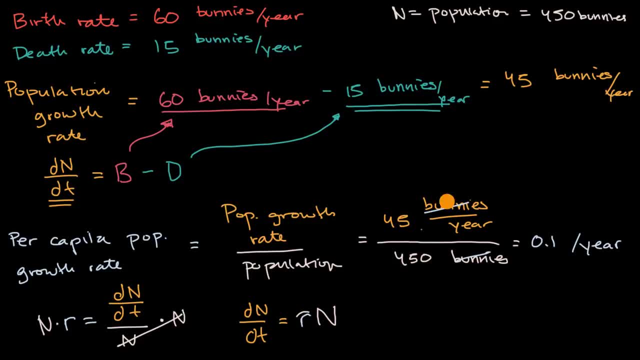 well, if you multiply the two, you'll know how much the whole population has grown. So if we didn't know these numbers and someone said, hey, well, actually we could think about this. Let's think about now a population of 1,000 bunnies. 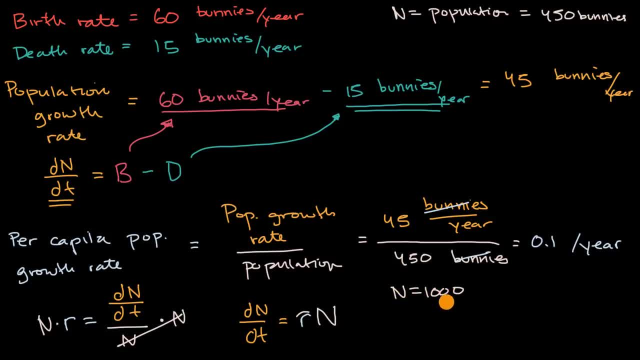 So if N was equal to 1,000,. and let's say they're the same type of bunnies that have the same probability of reproducing and the same likelihood. so we know that R is equal to 0.1, per year. 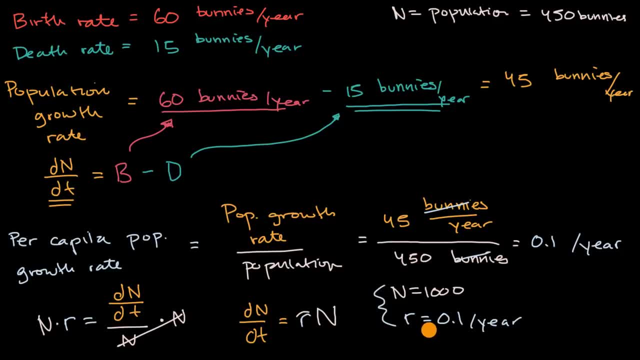 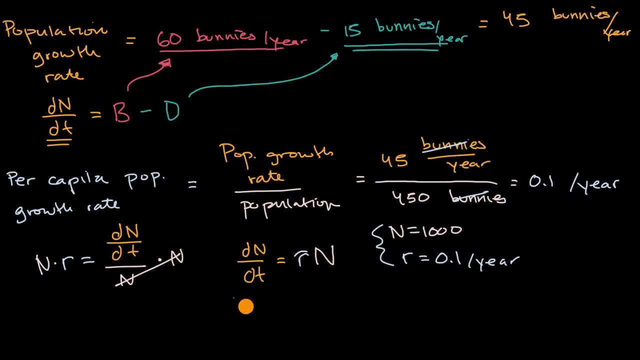 for this population of bunnies. what is going to be our population growth rate? Pause this video and try to figure that out. Well, in this situation, dN, dt is going to be our per capita population growth rate, so it's going to be 0.1 per year. 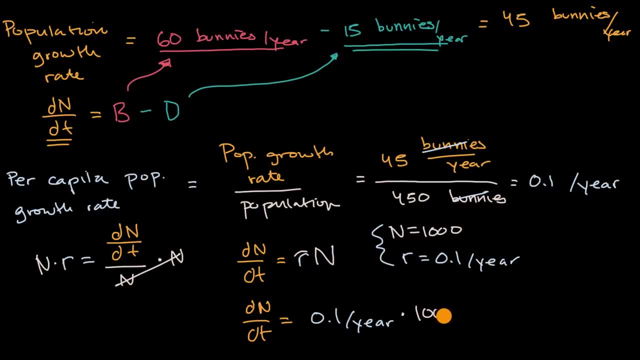 times our population, times 1,000 bunnies, Bunnies, bunnies. I'll keep my units here: bunnies. And so this is going to be equal to 1,000 times a tenth is 100, I ran that color. it's 100 bunnies, bunnies per year. 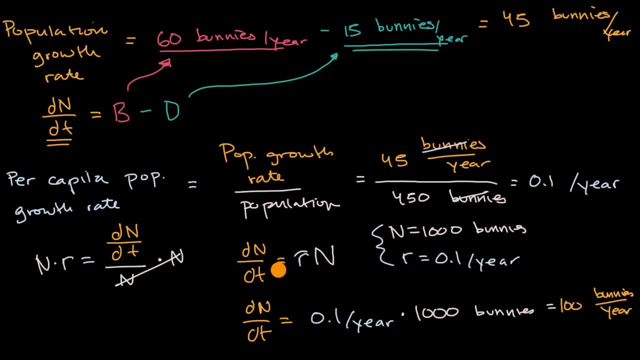 So hopefully you're getting an appreciation for why these types of formulas, which are fairly straightforward- they're using just a fancy notation- are useful. Now, this is also an interesting thing to look at, because even though that this is in fancy calculus notation- 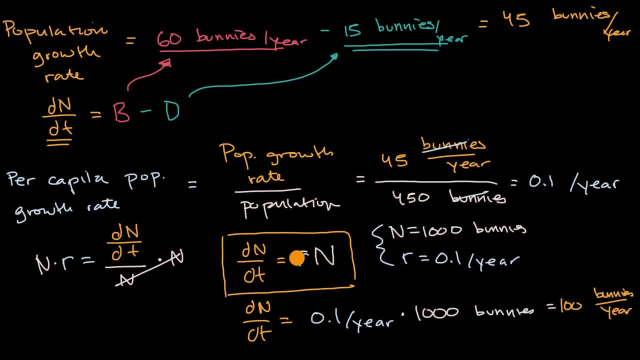 and they're saying that our rate of change of population is equal to R times our population. this is actually a differential equation. if you were to think about what this population, the type of population this would describe, this would actually be a population that's growing exponentially. 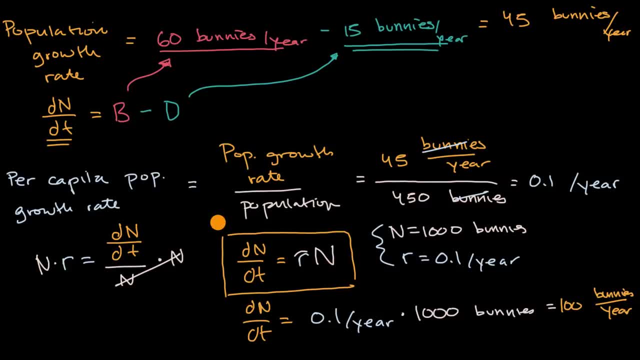 So this is often known as an exponential growth equation. Let me write that down: Exponential exponential growth. And in other, in your math classes, in your calculus classes or even in your pre-calculus classes, you will study exponential growth. 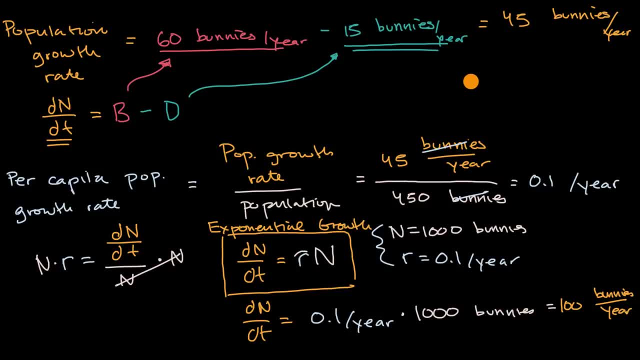 In a biology class. you're really just thinking about how to manipulate this a little bit. but just to give you a little sense of what's going on with exponential growth, if you have a population of bunnies with this type of exponential growth, 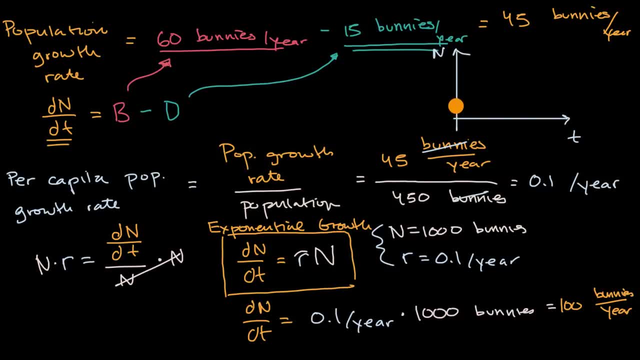 what is happening here. this is time and this is your population. So you're going to have some starting population here and it's just going to grow exponentially. And the higher the R is the steeper right, the higher the R is the steeper right.